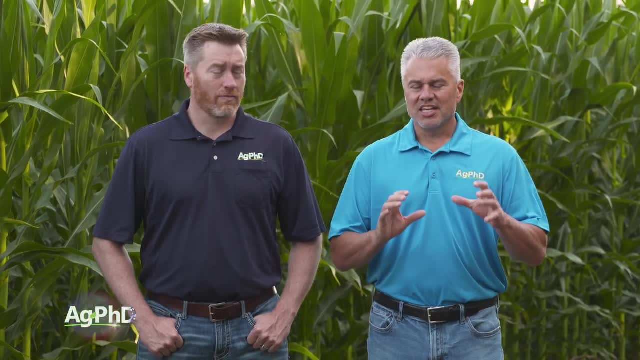 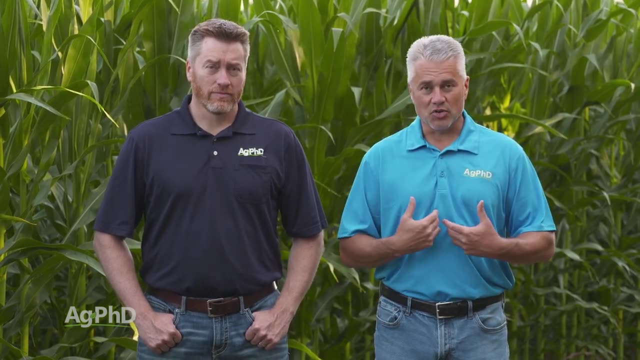 find most interesting about this overall is just that insects will have different forms at different times of the year and they can actually feed on our crops out in the field in different ways. So we just wanted to explain that a little bit today. Well, 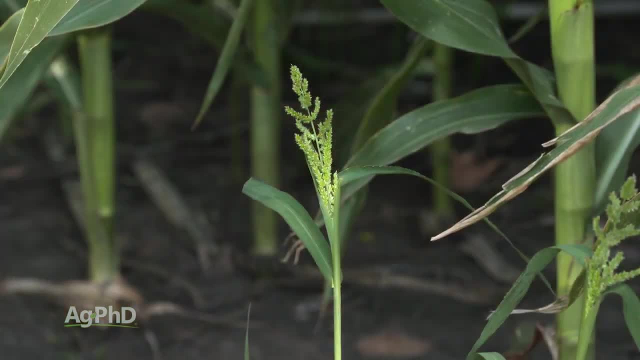 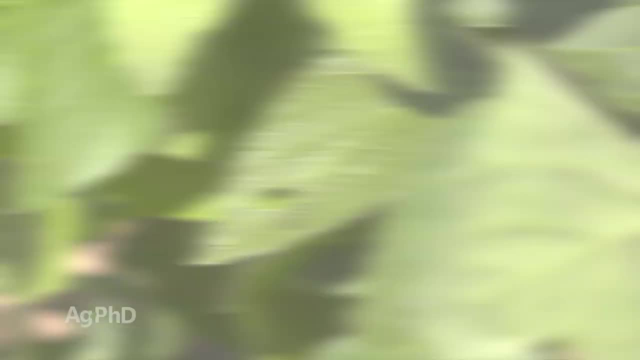 when we think about crops, their one goal in the year, or weeds, for that example, is to produce seed so they can live the next year. Well, the same thing is true with bugs, So you may see some bugs out there, right? 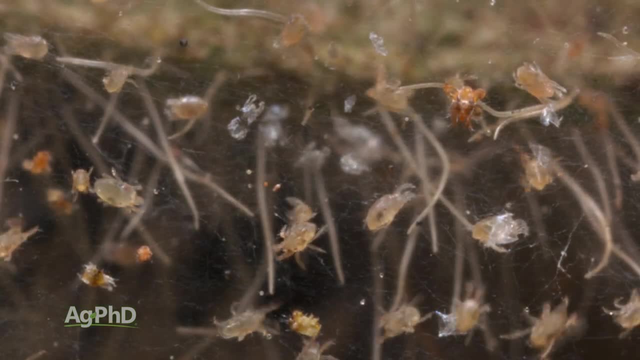 now, but are they going to live the next year? Well, are they going to lay eggs? Are they going to overwinter somehow, so they could impact next year's crop? So the damage may already be done for this year, and let's just 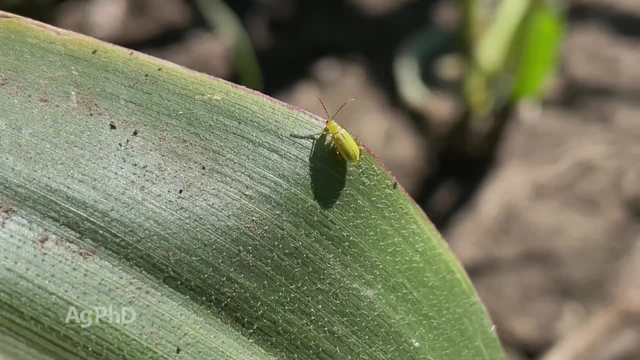 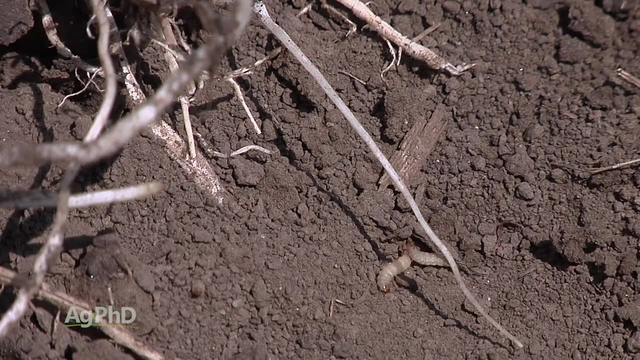 give you a few examples: Corn rootworm: When we think about corn rootworm larvae chewing on the roots of corn, well, that gets every farmer excited. but when you see these kind of harmless-looking little beetles that may do just a little bit of feeding, but generally, 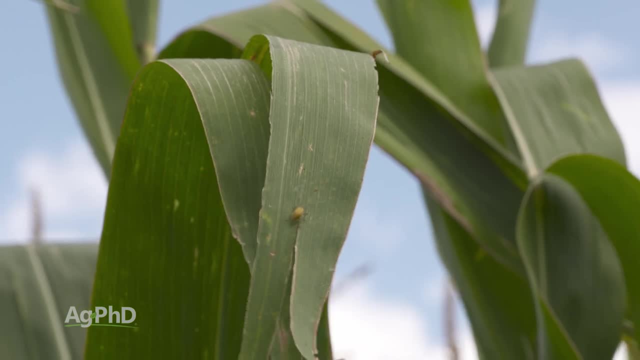 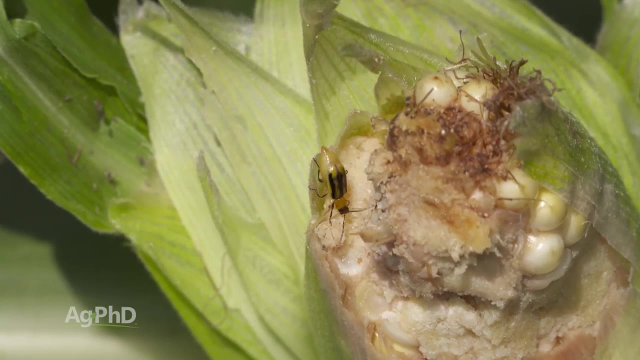 aren't a big problem. later in the season you think: well, that's no big deal, I don't have to worry about that. Those corn rootworm beetles are going to lay eggs in the field and next year those eggs can hatch attack next. 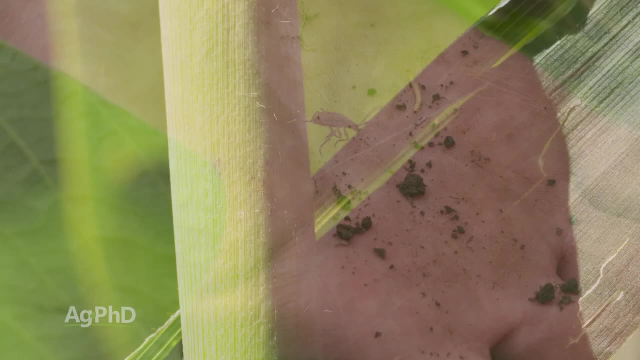 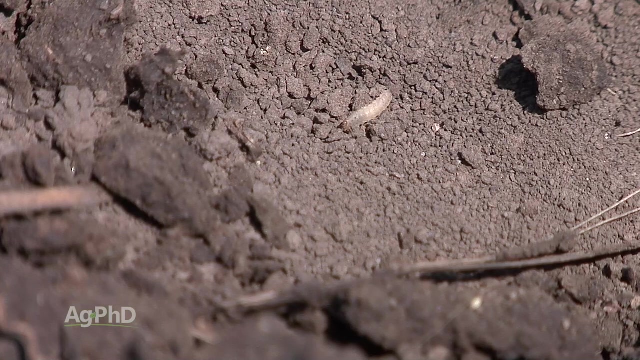 year's corn crop and you can have some big problems. So you may see something that looks pretty harmless now. it could be a big problem next year. Ok, Darren, just gave you the example of the youth or larvae stage versus the adult or beetle stage of one. 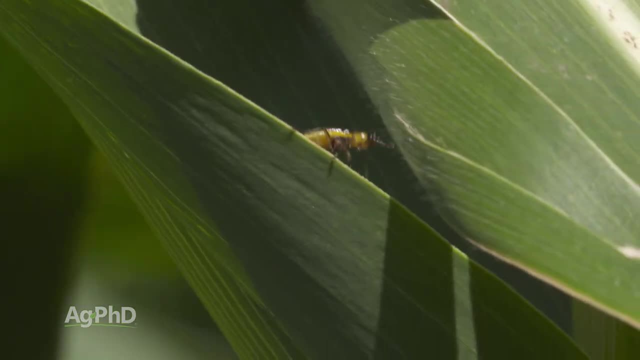 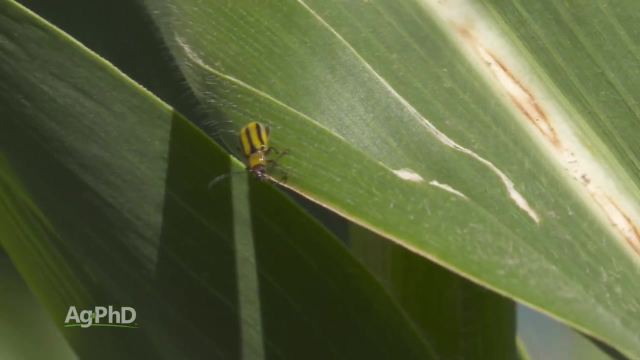 particular insect. Well, when you think about beetles, they can't fly very far, can't move very far or anything else. So typically when we have a corn rootworm issue, that's usually an isolated problem. So if it's in one field, how far can it really move? 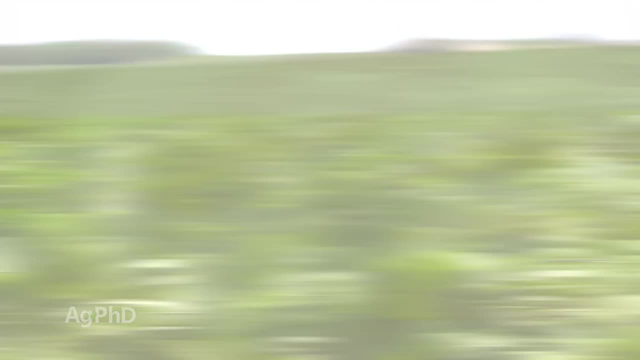 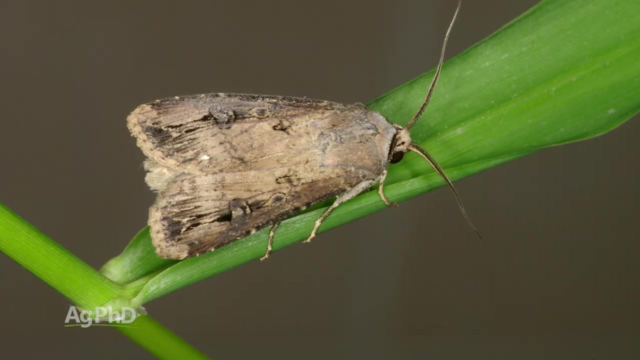 It could spread out just a little bit to some neighboring fields. that's probably about it. A different insect that I think about- from actually one of the first ones I was ever familiar with, was black cutworm, and what happens with black cutworm the adult? 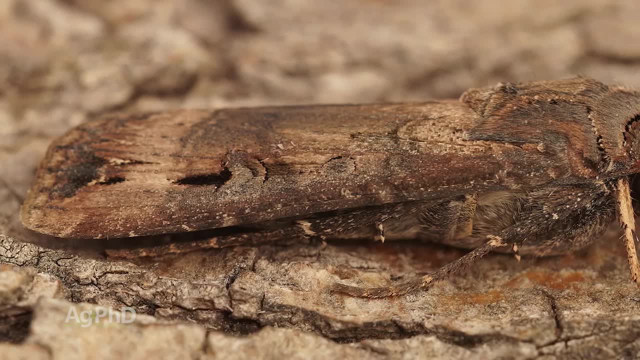 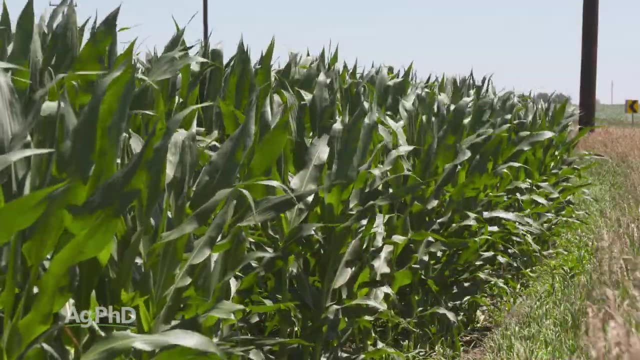 stage is a moth. So moths, they can move in some cases hundreds of miles, if not even thousands of miles. and so all of a sudden you say, oh, we've never had that problem. We've had that problem around here before, and the